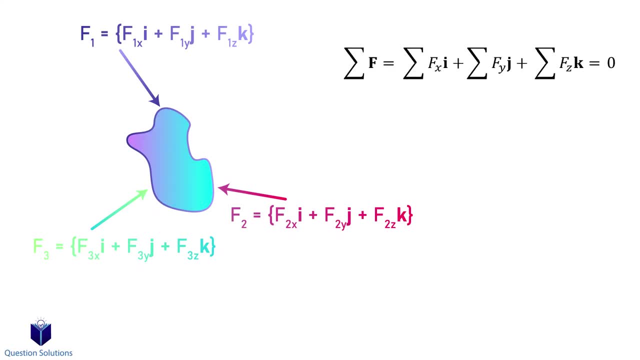 to stay in equilibrium, in other words not move, all the x components added together must equal zero. The same goes for y components and z components. The same is also true for moments. So if we calculate the moment about a point or an axis, the components must equal to zero. 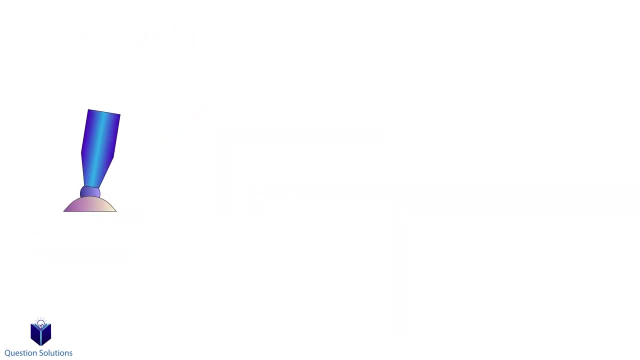 otherwise the object wouldn't be in equilibrium. Each object will have different supports and each support will be in equilibrium. Your textbooks will have a list of these, so please take a look. In addition to solve these problems, you must know how to express forces in Cartesian form. 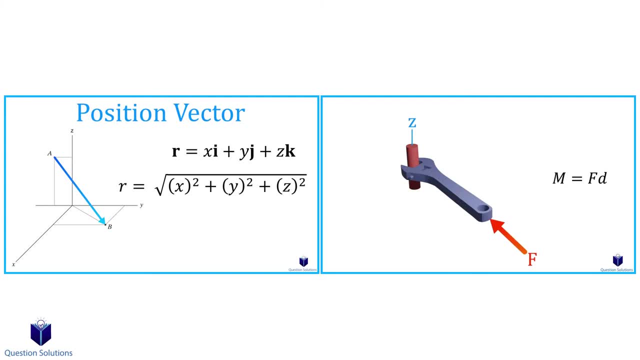 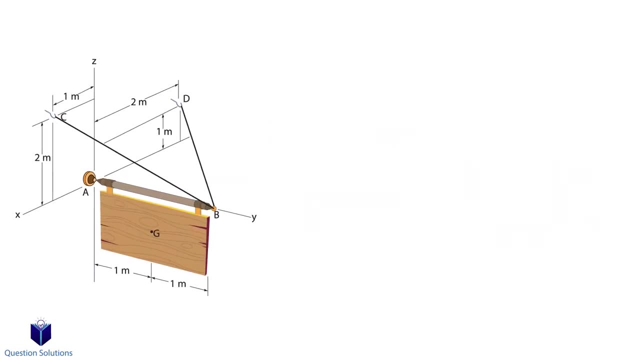 and how to find moments. If you need to refresh or forgot, please take a look at the description. Now let's get to some examples and go through how to solve them. In this problem, we need to figure out the reactions at the ball and socket joint. 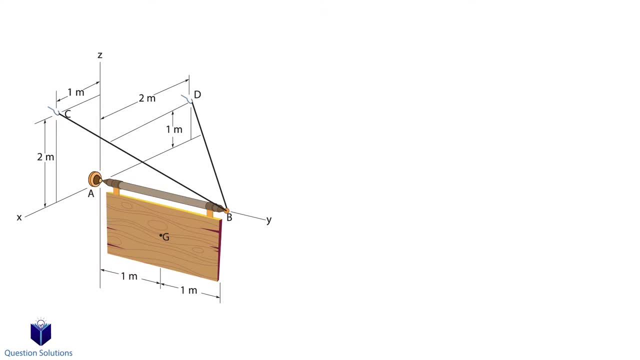 and the tensions in the wires. The sign has a mass of 100 kilograms, so the vector for weight will be straight down and it will only have a k component. So now we need to think about the support reactions. At A we have a ball and socket joint. that means we will have three reactions. 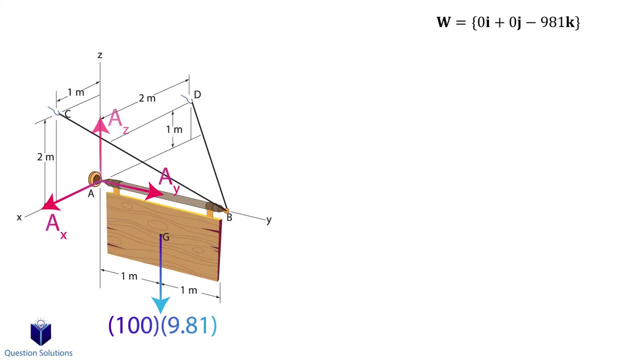 one in the x direction, one in the y direction and another in the z direction. We will assume that these reactions face the positive x, y and z axes. Since the ball can rotate inside the socket, no moment reactions will be created about point A. 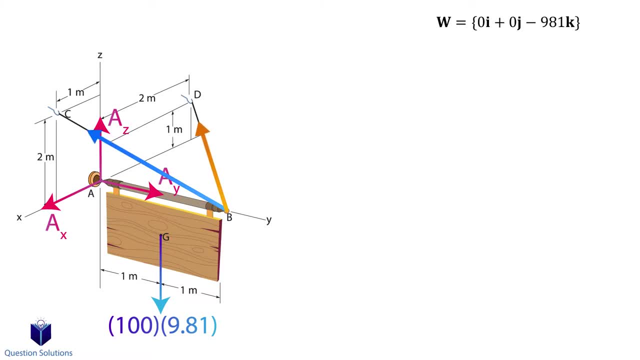 For the two wires. we will have two forces going from point B towards C and D. We have to express the force in the wires in Cartesian form. To do that we first need two position vectors: from B to C and B to D. 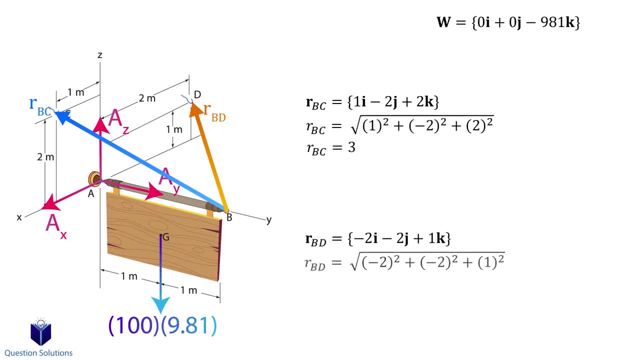 Next, we need to find the magnitude of each position vector. Now we find the unit vector by dividing each term in the position vector by the magnitude. Lastly, we can express each force in the wire. So we're just multiplying the magnitude, which we don't know yet, by the unit vector. 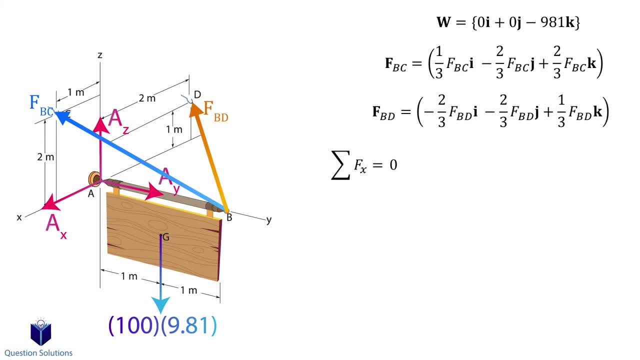 OK, now we can equate the components. So what we are saying is that for this sign to not move around, all the forces in the x direction has to add up to zero. The same for y direction and the z direction. Let's start with the x-axis forces. 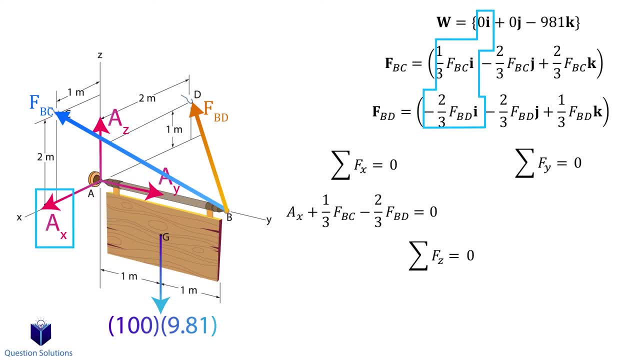 So we have the x-axis reaction at A and then the i component of wire B c and the i component of wire B d. All of that added together has to equal zero for this object to stay in equilibrium. Next, y-axis forces. 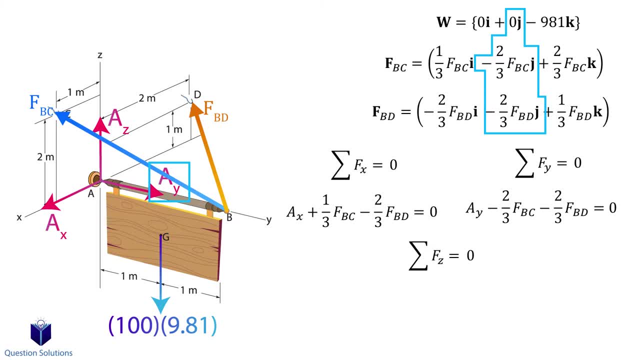 It's the same as before, but now we're just looking for forces in the y-axis. Lastly, we have the z-axis forces. Don't forget the weight of the sign. Notice how we have three equations with four unknowns, So we need one more equation. 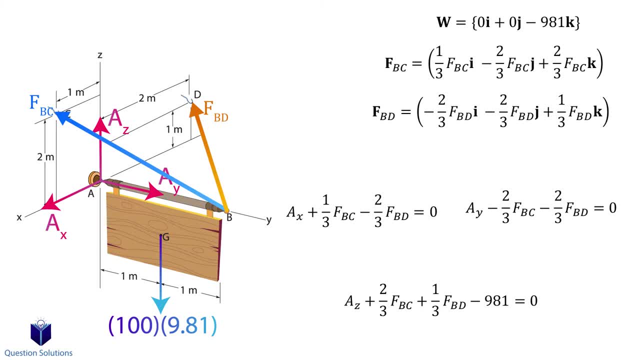 That's going to be a moment equation and we will write it about point A. We will first calculate the moment created about point A by the two wires. To do that we need a position vector from A to B. That's where our two wire forces start. 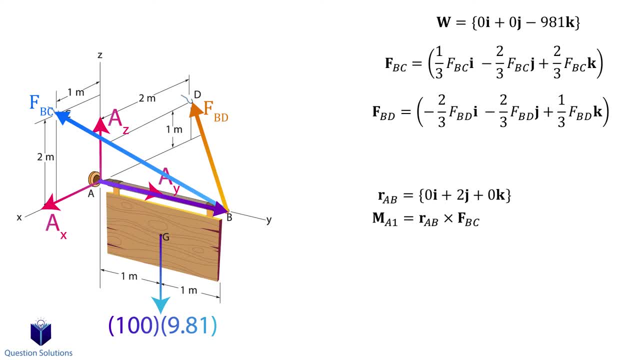 So let's calculate each individual moment created by the wires. First wire BC. Next we calculate the moment created about point A by wire BD. Now we need to figure out the moment created by the weight about point A. For that we need a position vector from A to G. 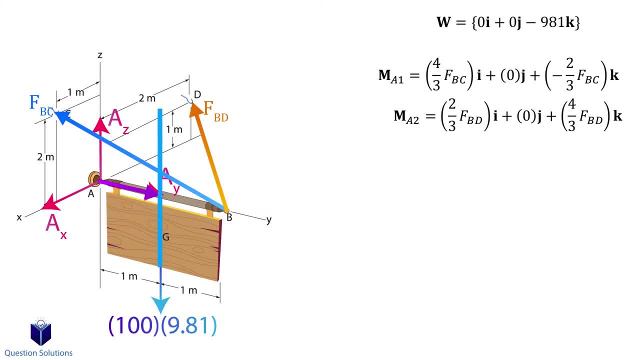 We actually only need a position vector to the vertical distance of point G along bar AB, Because its line of action crosses the bar. Let's calculate the moment created about A by the weight. Now, for the object to stay still, all of the moments added together must also equal zero. 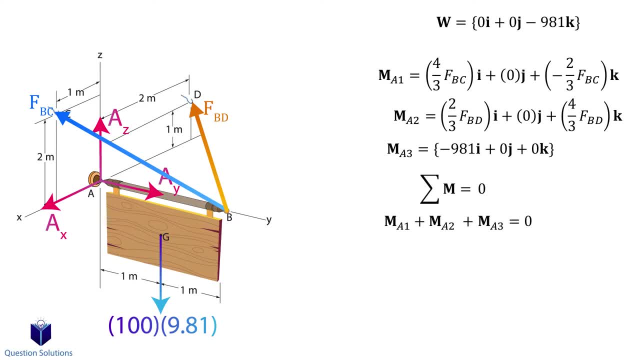 Also keep in mind that since we wrote our moment equation about point A, the reactions at A won't create any moments. Now, just using our moment equation, we can actually figure out FBC and FBD. All we're going to do is equate the components to zero. 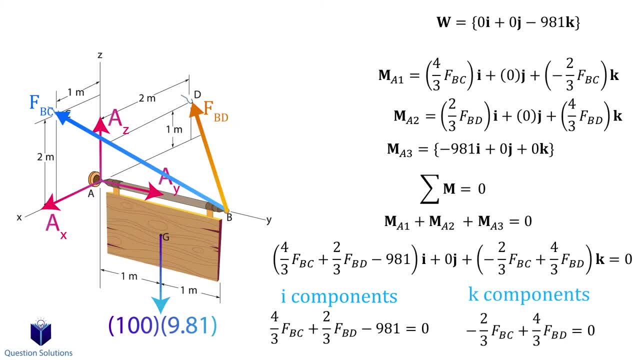 So we equate all the I components to zero and all the K components to zero. components to zero. We don't have any j components, so we don't need to worry about it. Solving the two equations gives us the forces in the two cables. Now, using the values we just found, 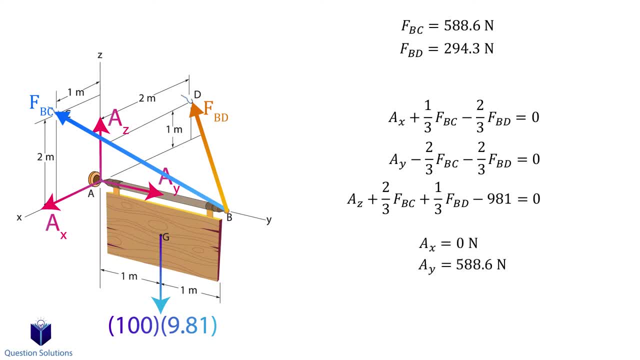 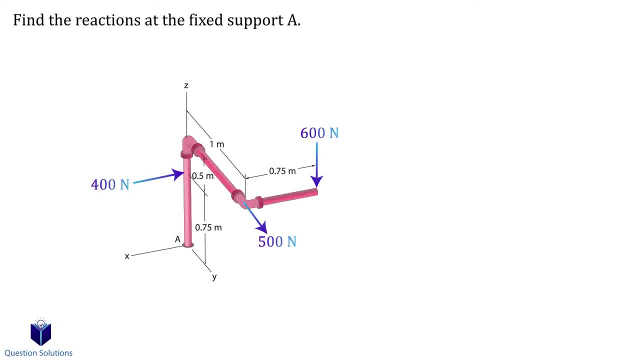 we can solve the other three equations for the unknown reactions at A. Those are our answers. Let's take a look at this problem where we need to find the reactions at the fixed support A. The first step is to express each force in Cartesian form: The 400 N force. 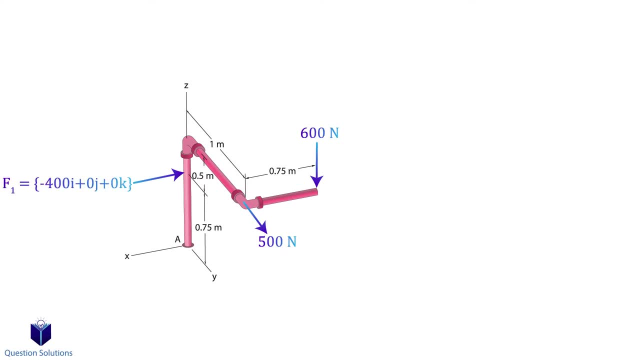 is along the x axis, so it'll only have an i component. It's negative because it's facing right and our x axis faces left. The 500 N force is along the y axis, so it'll only have a j component. And lastly, the 600 N force is along the z axis, so that will only have. 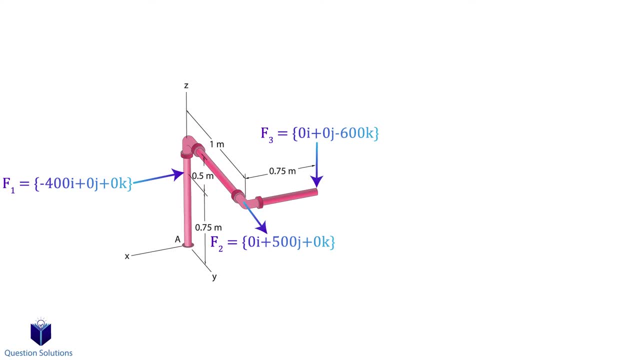 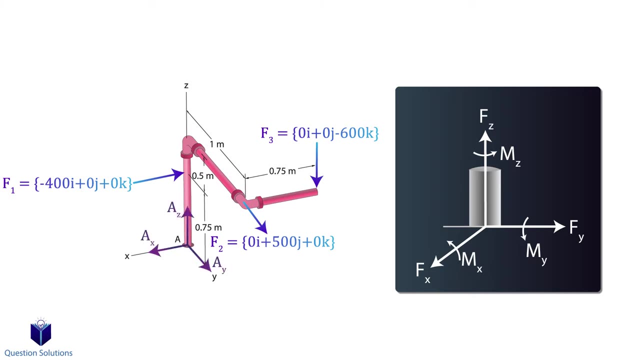 a k component. It's negative because it's downwards, while the z axis faces upwards. Now, since it's a fixed support at A, we know there'll be six reactions: Three forces and three couple moments about each axis. So the first step is to express each force in Cartesian form. The first step is to express 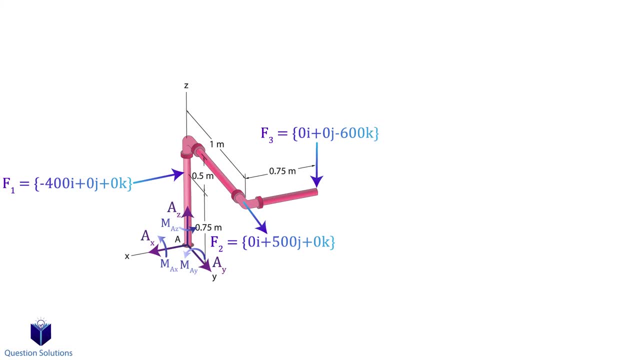 each force in Cartesian form. To figure out the three force reactions, we just need to write three equilibrium equations, one for each axis. Let's start with the x axis forces. We only have two forces: the x reaction at A and the 400 N force. Next, y axis forces. 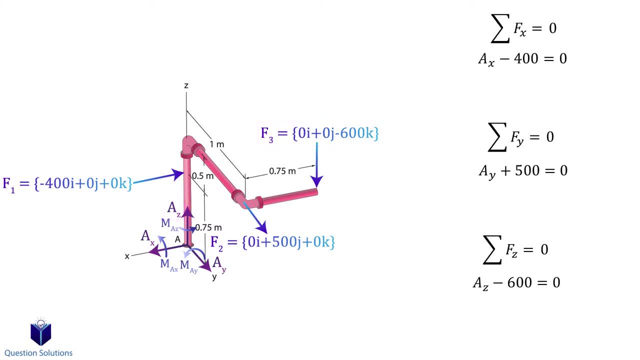 Lastly, is the z axis forces. Now let's solve all the equations to get the reactions. Notice that we got a negative value for Ay. All it means is that while we assumed the reaction at A to point in the y direction, In reality it's facing the other way. 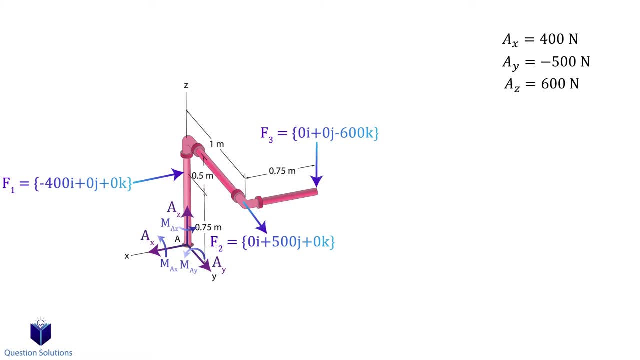 Now we need to figure out the moment reactions about point A. To do that, we need to calculate the moment created by each force about point A. So first we need position vectors from A to where each of the forces are being applied. from Now, let's calculate each moment created. 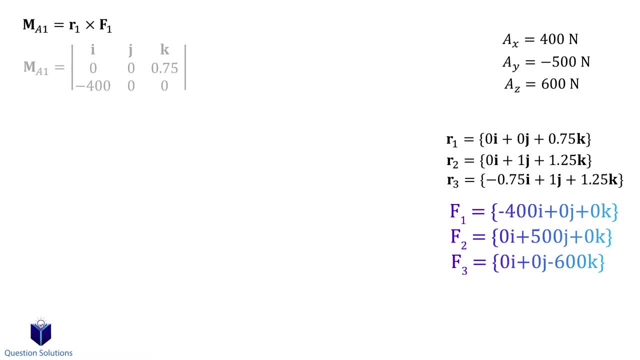 about point A by each force, starting with the 400 N force, Next the 500 N force, Lastly we have the 600 N force, Next the 500 N force, Lastly we have the 600 N force, Next we have: 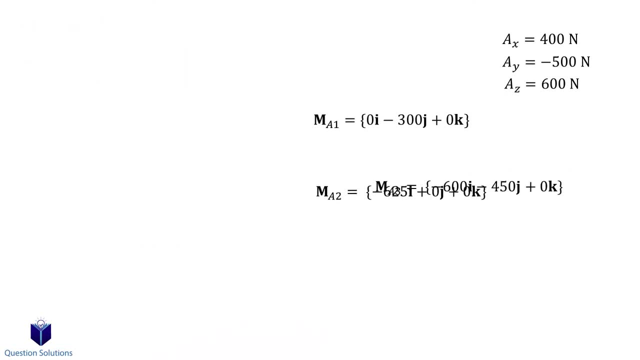 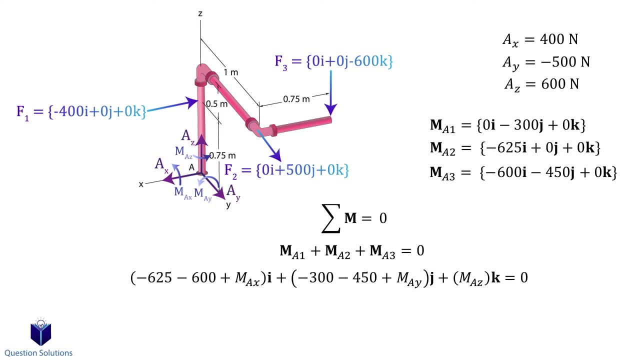 the 600 N force. Now all the moments added together must equal zero, otherwise the object would be moving. Step 4, we also include the reaction moments at point A as well. Note that for the moment, about the z axis, we only have reaction in this regard. 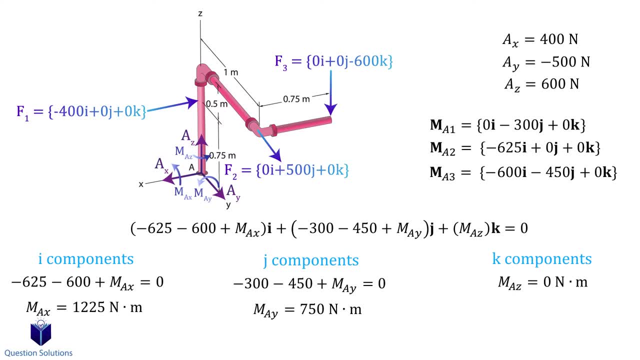 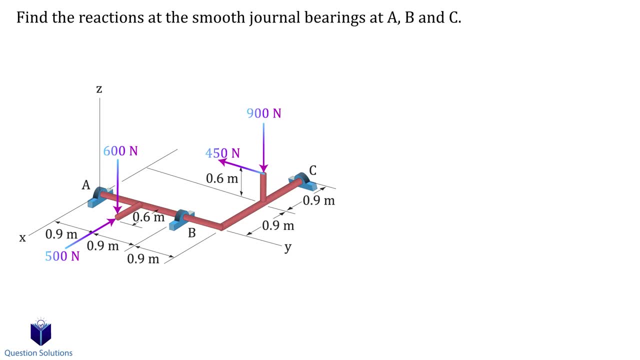 Now we can equate each of the components to zero. Solving gives us our answers In this question. there are three smooth journal bearings at A, B and C. So this is b of the proposals You can hip pots into E. Make sure that were in the correct谷 conclusion. 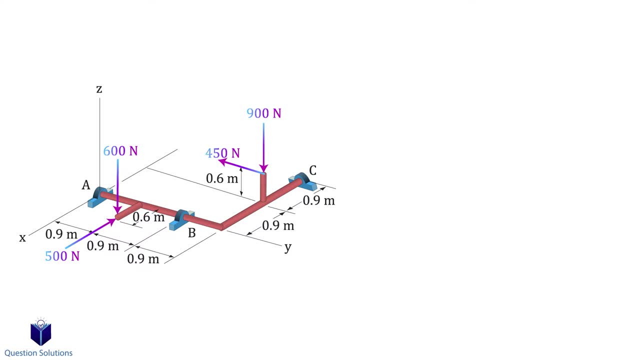 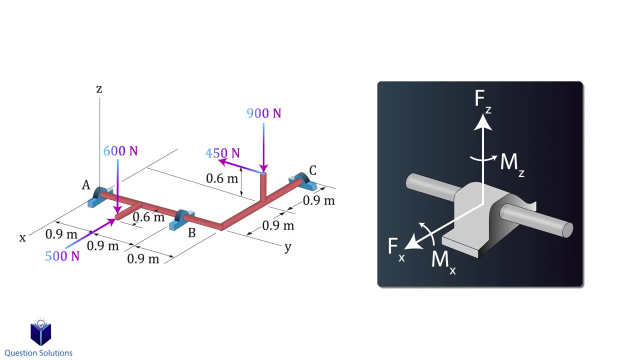 and we need to figure out the reactions. So our first step is to figure out what type of reactions are created at the bearings. Normally, smooth journal bearings will have two reaction forces that act perpendicular to the shaft and two couple moments. However, the couple moments are usually not applied if the object is supported at other. 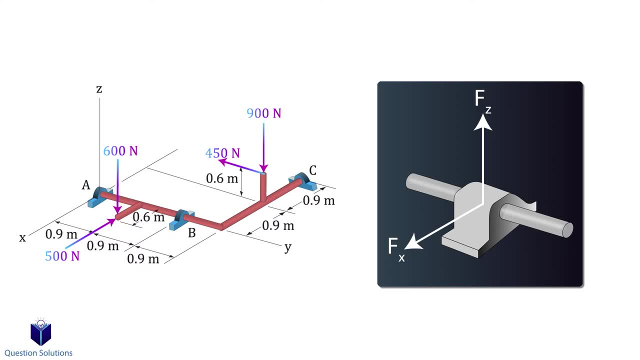 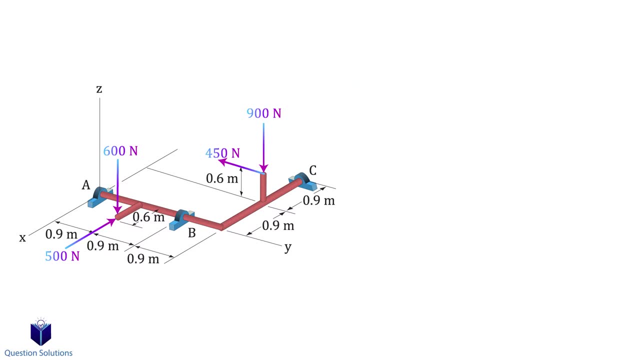 places. This is the case with this example. Since we have three supports, the couple moments will not be applied. So each smooth journal bearing will have two reactions that are perpendicular to the shaft. At A, we would have a reaction in the X direction and the Z direction. 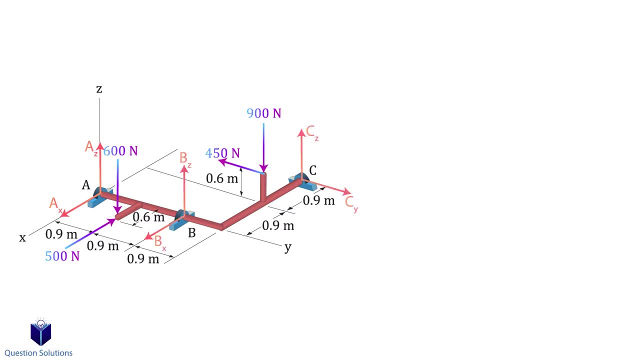 B would also have the same two reactions. At C, we would have a reaction in the Y direction and a reaction in the Z direction. I just want to show you why there won't be a reaction in the Y direction at A and B. 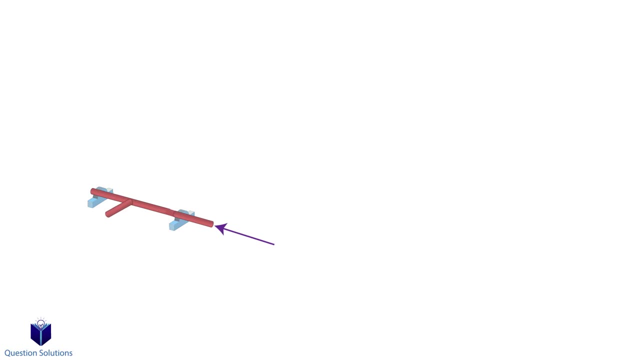 Imagine we remove this part and we push on the rod from this side. Notice how it can slide through the support. That means the smooth journal bearing cannot apply a reactive force to stop it from going along the Y axis. Now if we put back the section we removed before the bearing at C would prevent the 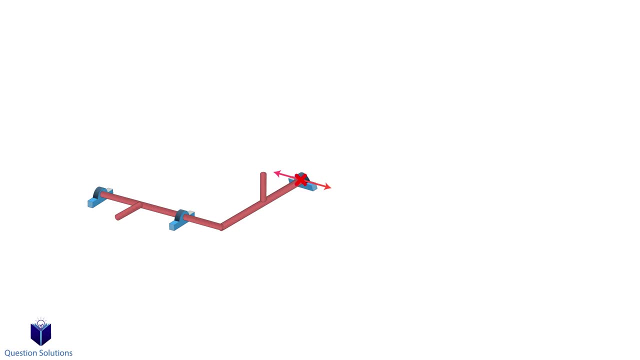 whole piece from moving in the Y direction, because here the bearing stops the movement in the Y direction while not applying a reactive force in the X direction. This is also why moments aren't created, because the object is supported at multiple places. Now let's write an equation of equilibrium for the Y axis forces, since we would only 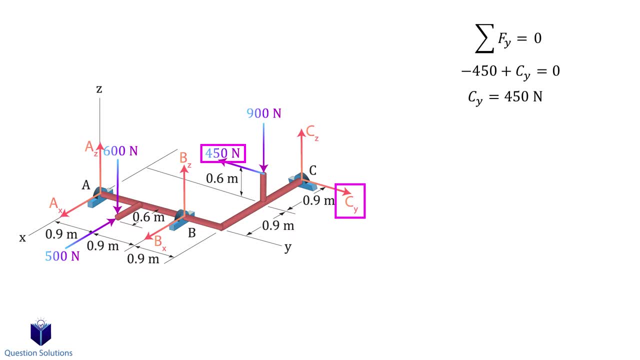 have one unknown. Solving gives us the Y reaction. Solving gives us the Y reaction. Now how can we find the Z reaction at C? The easiest way is to write a moment equation about the Y axis. Only two forces create a moment about the Y axis, in addition to the Z component at C. 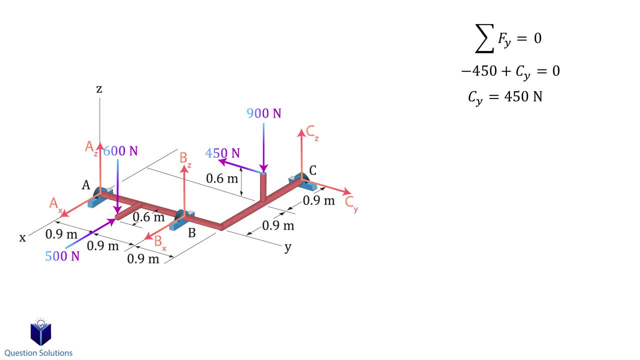 Since we're going to figure out the moment using a scalar method, so just multiplying forces by perpendicular distance instead of the cross product. we have to be careful about our positive and negative signs. To figure out the positive and negative signs, make sure to use the right hand rule. 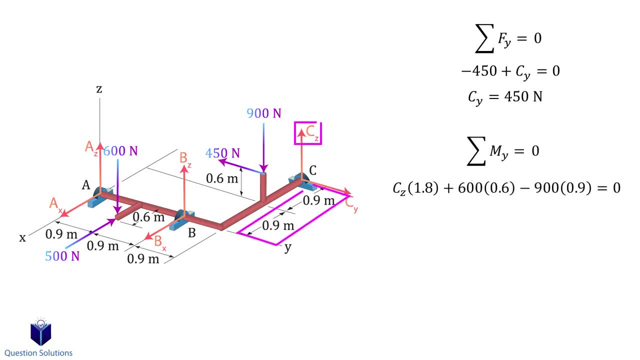 So we have the reaction in the Z direction times the perpendicular distance to the Y axis, then we have the 600N force times 0.6 meters and lastly we have the 900N force times 0.9 meters. 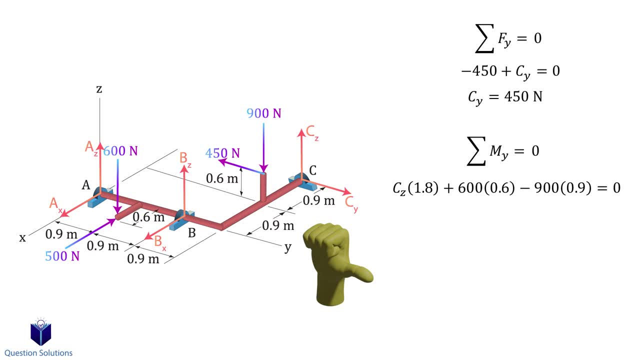 The 900N force causes a clockwise moment, so it'll be negative. Now let's solve. So we figured out two of the reactions. let's figure out the other four. We will write an equation of equilibrium for the X axis forces.